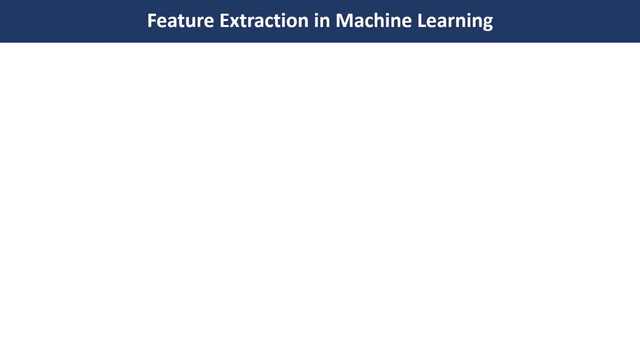 Hello everyone. today we are going to discuss about the feature abstraction in machine learning. First we will understand why the feature abstraction is required. Feature abstraction is usually used when the original raw data- original raw data- is very different and we cannot use this raw data for our machine learning modeling. Then we perform the feature abstraction or feature. 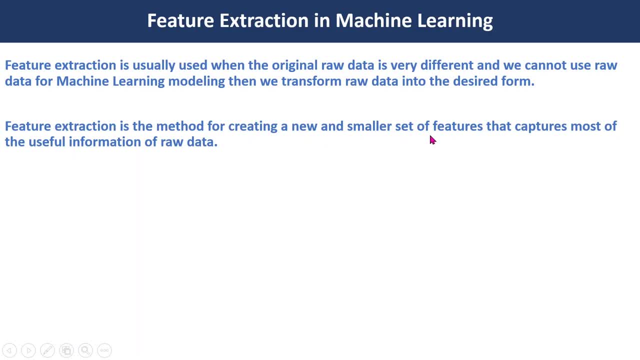 abstraction is the method for creating new or a smaller set of features that capture most of the useful information of that raw data. As we know, in the real world machine learning problem we rarely use the CSV data, So we have to extract the some useful information from the raw data. Some of the 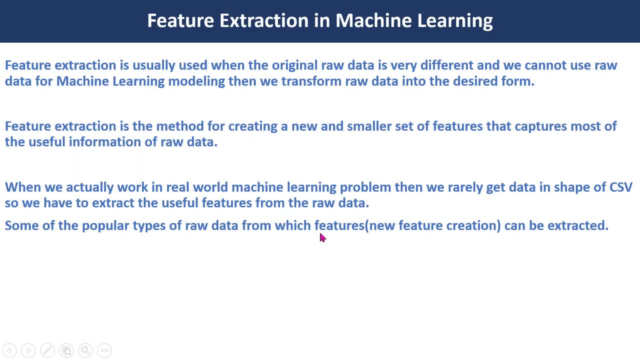 different popular type of the raw data from which features can be extracted. or we can create a some new data. So we have to extract the some useful information from the raw data, So we have to new features. So these are the some raw data which we cannot like directly use for our machine. 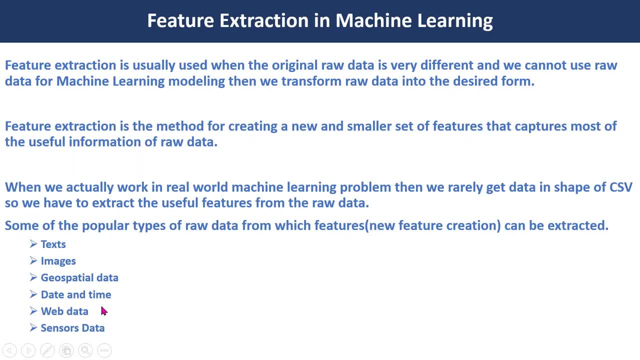 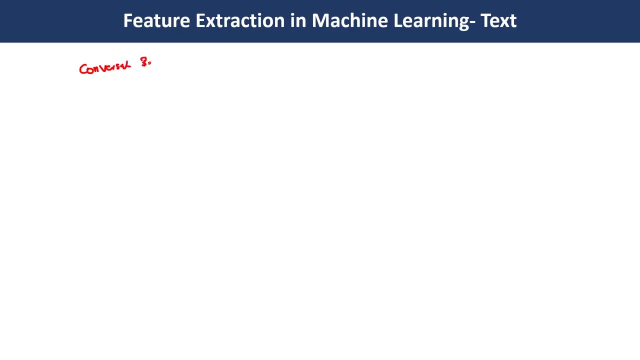 learning modeling. So we will discuss one by one. First one is your test Let's. I am going to create one conversational bot, So for that we would need some data for our machine learning modeling to to make this conversational bot, Because this is a conversational bot. 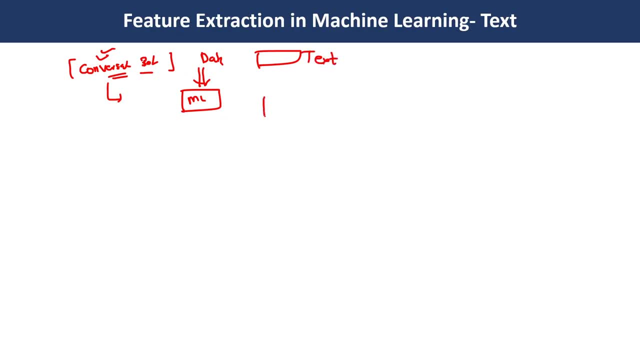 so we would need some text data. So, as a machine, this is your machine. So machine doesn't understand this test data Like. so we have to convert this test data into a vector or into a matrix. So to conversion from text to vector or matrix by using some technique or method. 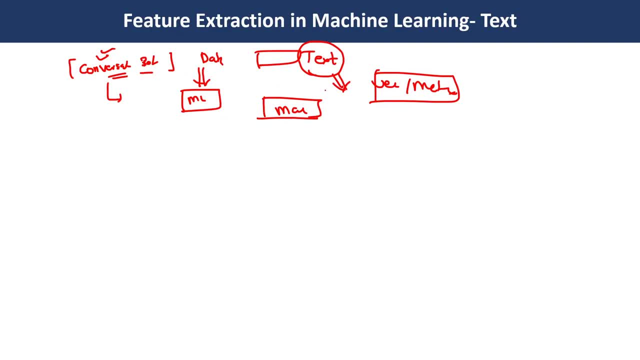 that is called as a feature abstraction from the text data. Where we will use a feature abstraction method, We will use different technique, like bag of bars, like your tf-idf. There are different, different methods we used to perform for text data pre-processing. We will cover all these. 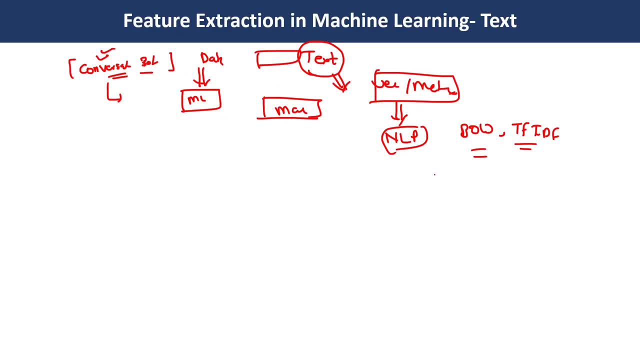 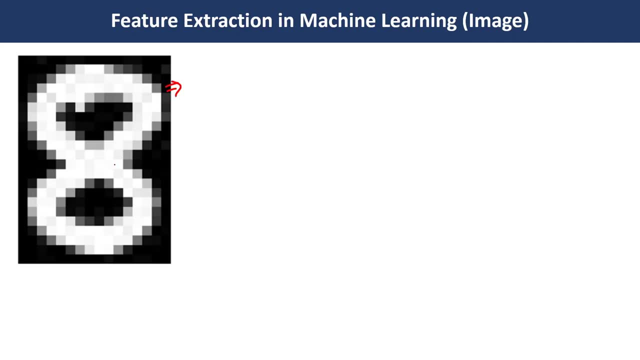 steps in natural language processing in NLP. And second one is your image. Like this is your image As a human. we are able to understand that this image is made of a small, small pixels, We are able to understand. But if I will feed this image into a computer, computer will not be able. 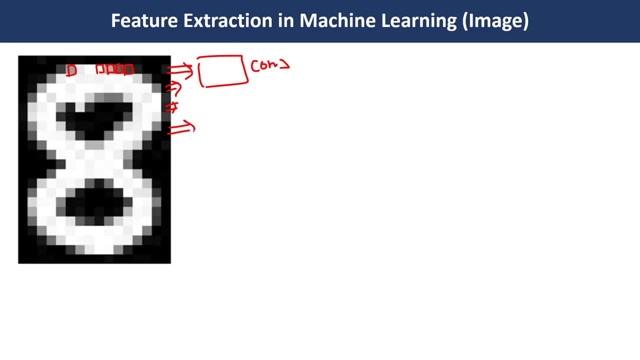 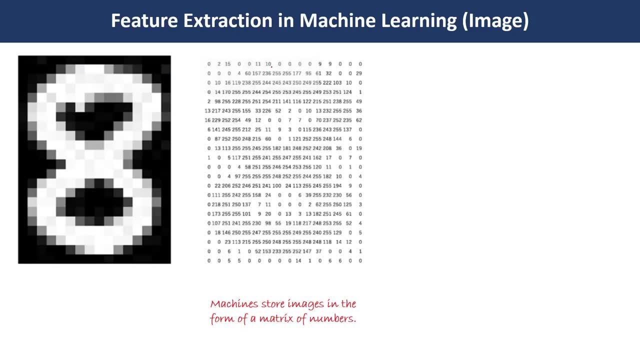 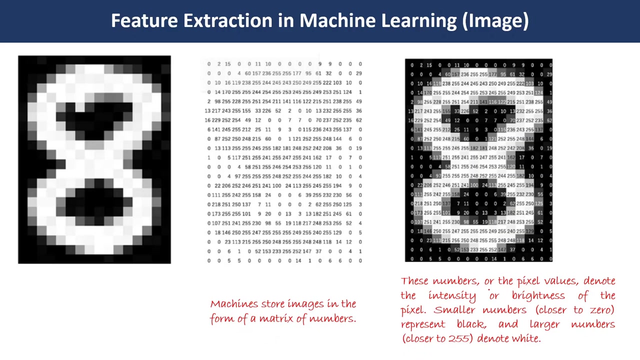 to understand. So for that we have to convert this image into a matrix or into a vector. So what we used to do, we use this particular matrix Machine: store images in the form of matrix or a number, So after that we can see that these numbers or a pixel value denote the intensity of the brightness. 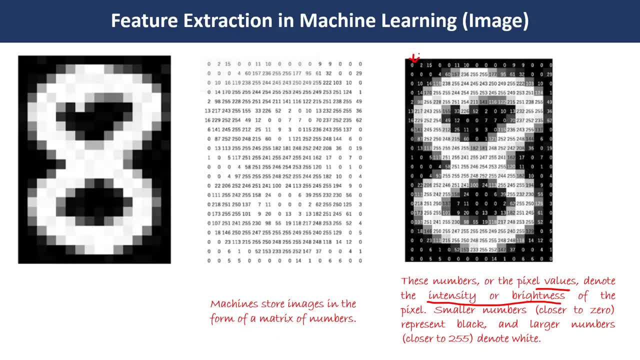 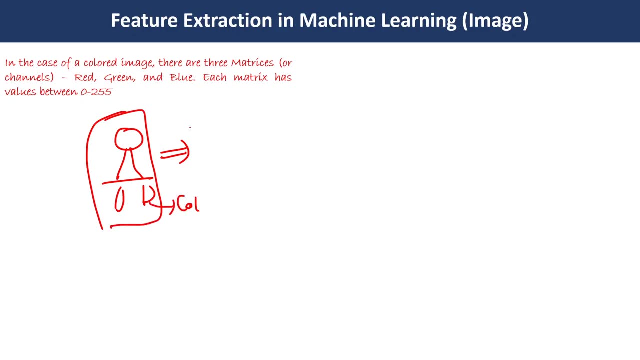 Right. Whenever we have, like, the low value, it means that is a dark. Whenever we have a high value, it means it is a light, It means brighter And in case of the colored image, this is a human image and this is a colored image. So in a colored image we have three channel. 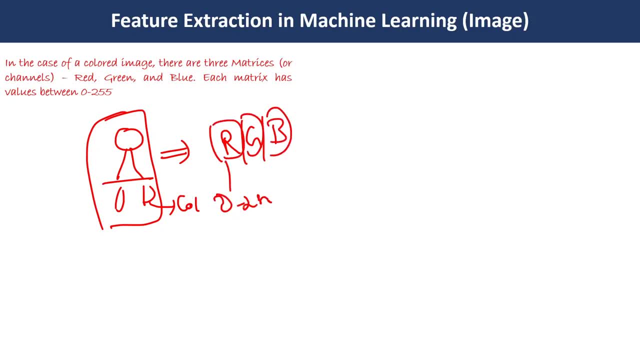 And each channel has 0 to 255 pixels. So we have to convert these images into a matrix as per our requirement. All these things I will cover in our computer vision playlist, So you can understand that I want to create a one classification model for images. So in that case we have to convert: 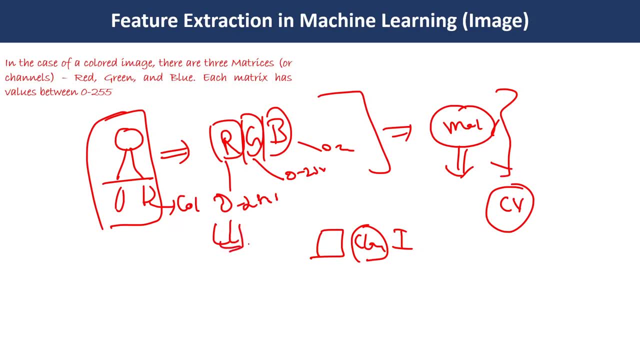 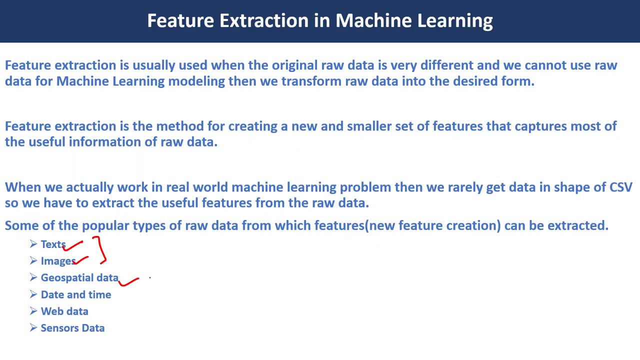 all the images which we are going to use to train our model into a matrix. Both we have covered. Third one is your geospatial data. So geospatial data we normally used to get in the PDF format In some, like your, in the 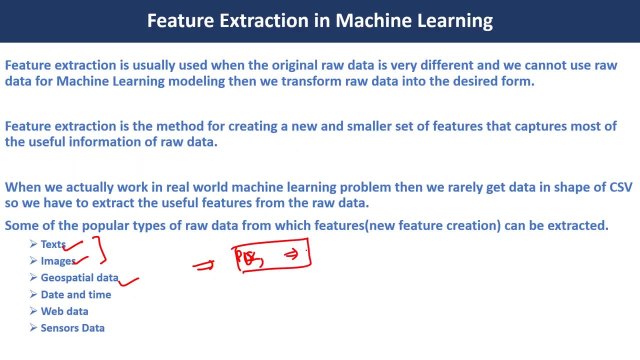 different, different format. we used to get the this type of the data. So let's, we want to create the weather forecasting. In that case, probably we would need some geospatial data. So let we want to extract some geospatial data from the data. So let's, we want to extract some geospatial data. 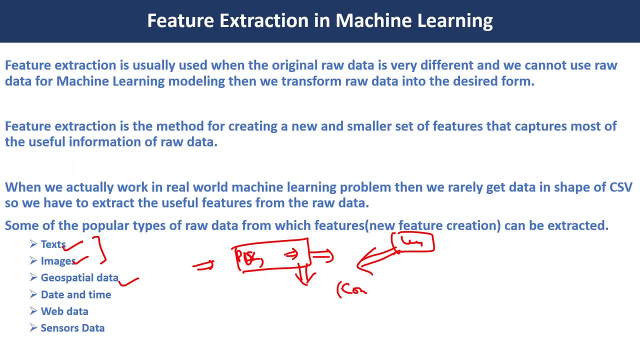 So, let's, we want to extract some geospatial data. So, let's, we want to extract some useful information from this PDF, like your: what is the coordinate of that particular location? what are the images of that particular location? So different, different type of the information we use to extract from this PDF.